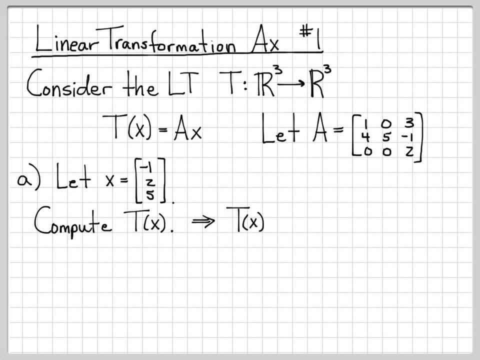 So that's almost trivial To compute t of x. we write down what t of x is equal to. It's equal to ax, which for this particular example is equal to the matrix A times the vector x. The vector x is a negative: 1,, 2,, 5.. So if we write this out, we know how to take a vector. 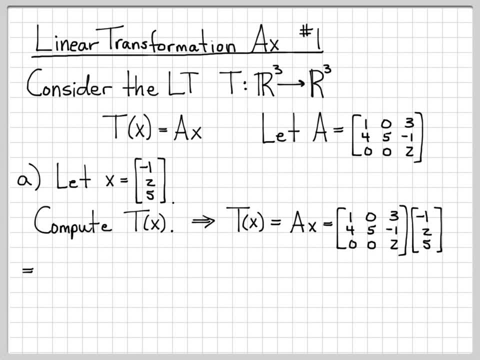 or I'm sorry, a matrix times a vector. each column of the matrix gets weighted by the corresponding entry of the vector. So this is going to be equal to the first column of A times the first entry of x, plus the second entry of x times the second column. 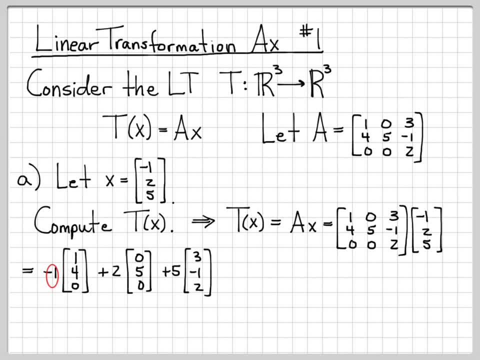 of A plus the third entry of x times the third column of A. And then we know how to do scalar multiplication: A negative 1 times that first vector, just changes the sign of every entry. So anything It turns into a negative 1, a negative 4,, 0. 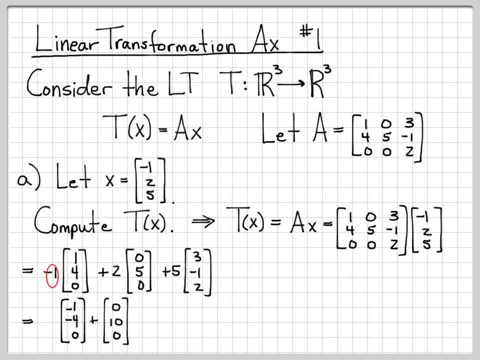 2 times. the second vector is just 2 times every element. So we have 0s in the first and third entries And 2 times 5 is 10 in the second, And then 5 times the third turns into 15, a negative 5, 10.. 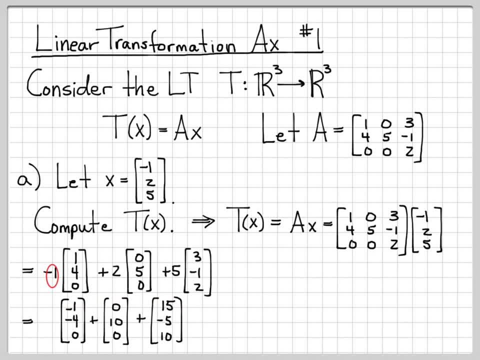 And then this is just vector addition. We just add all of these element-wise. So a negative 1 plus 0 plus 15 turns into 14.. A negative 4 plus 10 minus 5 turns into 1, because that's a negative 9 plus 10 is 1.. 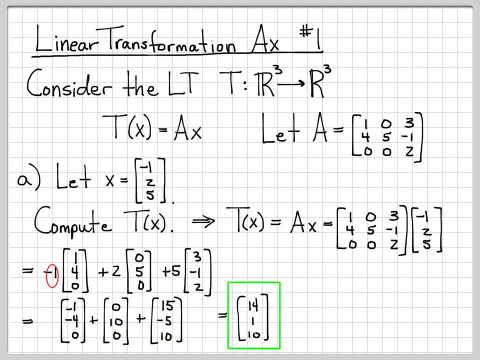 And the very last row: 0 plus 0 plus 10 is 10.. So we have computed the transformation of the vector x when x is equal to a negative. 1,, 2,, 5 for the specific case where our linear transformation is described by this matrix. 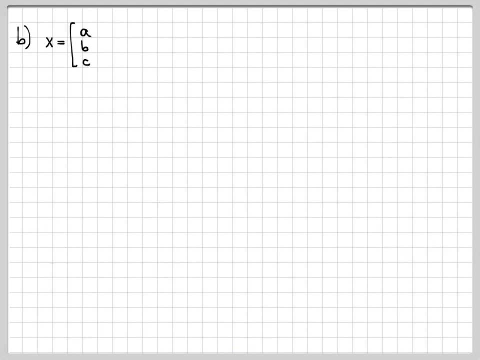 vector product. Let's do another example. In this example it's the same type of thing. We're going to also be considering The transformation t of x, where t of x is a of x, But in this case x is equal to the vector a, b, c. 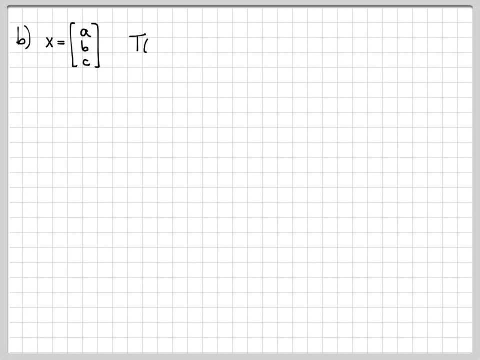 So we're just replacing a concrete instance with this variable a b c vector. So t of x is still equal to x, But now a is the same And x is now a b c. Well, I'm going to do the math. the exact same way. 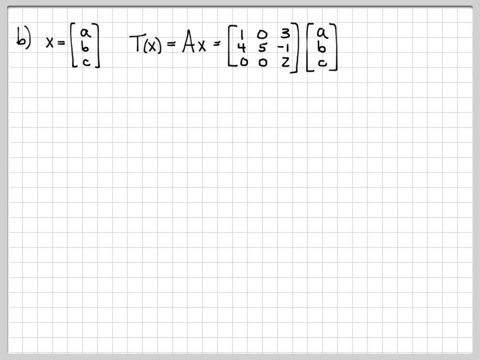 I'm going to have a times the first column plus b, times the second column, plus c times the third column, So I can go ahead and write that out. This is just the definition of matrix vector, Vector product. Each column of a gets weighted by the corresponding entry in the vector b. 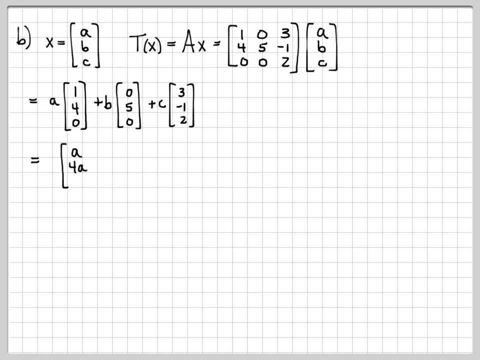 And then I can go ahead and multiply this out a times. that first column is a, 4a- 0.. This one is 0,, 5b, 0.. And the final one is 3c, a, negative c, 2c. 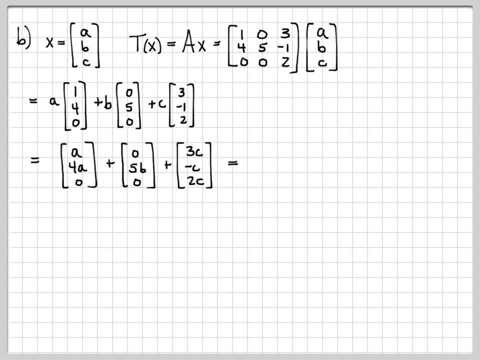 If I add all these up, do vector addition, I'll get a plus 3c, I'll get 4a plus 5b minus c And the final row is 0 plus 0 plus 3c. So I'm going to do vector addition. 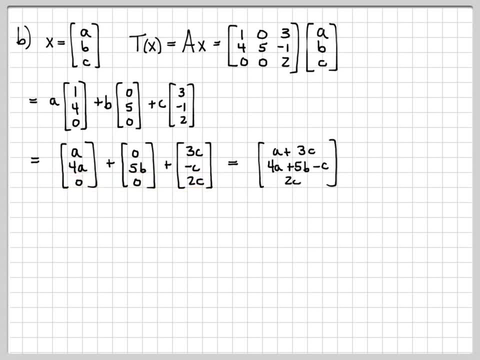 I'll get a plus 3c, I'll get a plus 2c, And this is my answer. This is the transformation of the vector x when x is equal to a, b, c And when the particular linear transformation we're looking at has a matrix representation. 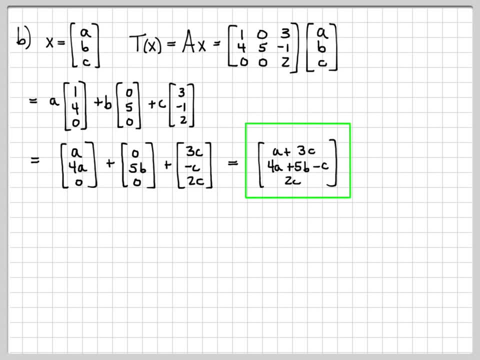 given by the matrix a. So we've completed this problem. We've looked at the linear transformation of two different vectors under the same linear transformation, a of x.